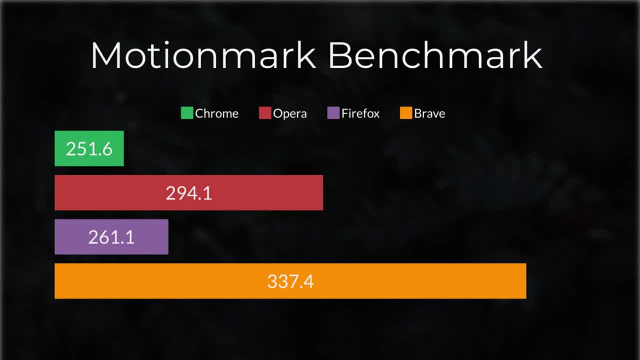 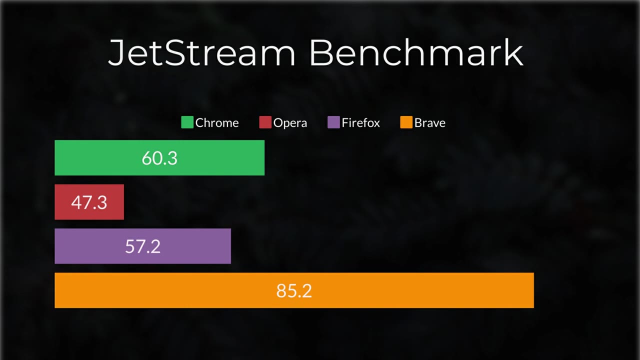 and Opera came second. MotionMark is a graphic benchmark that measures the browser's capability to animate complex scene at target frame rate. Jetstream benchmark scores focus on browsers that quickly start up, execute code quickly and run smoothly. Brave has the highest score, beating other browsers by a considerable margin. 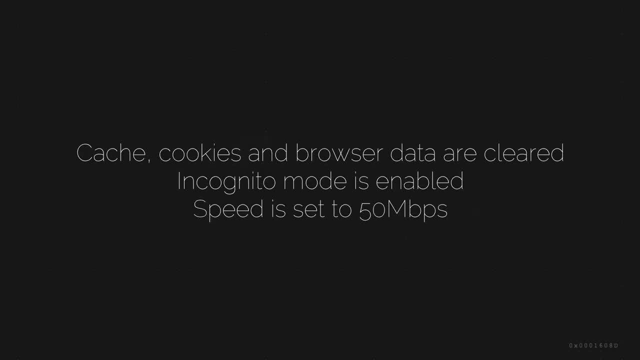 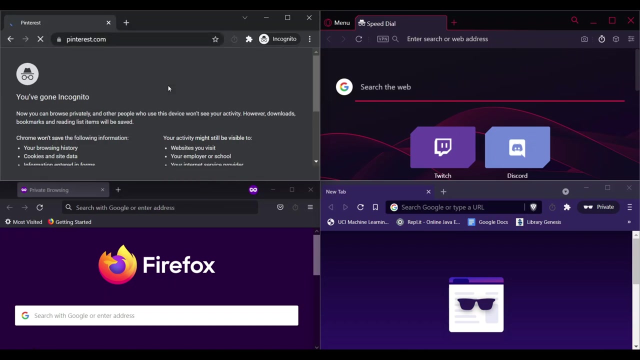 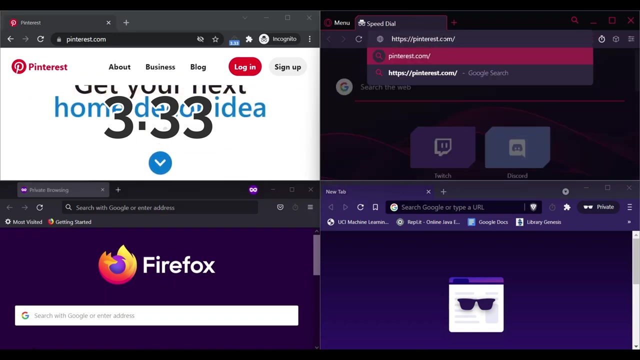 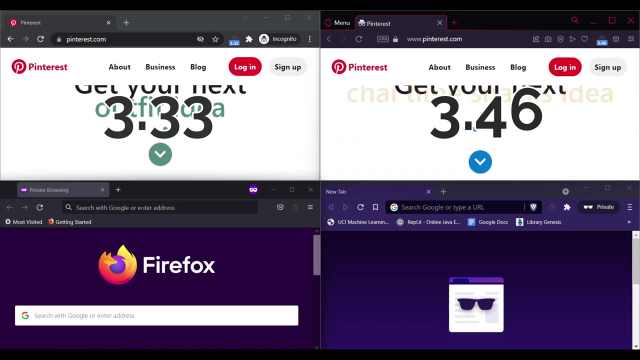 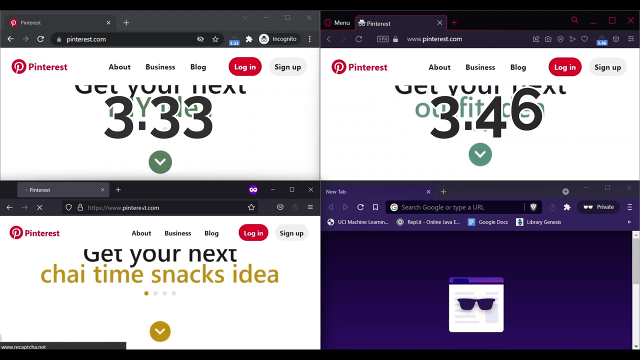 Next is the speed test. Cache cookies and browsing data are cleared, Incognito mode is enabled and speed is set to 50 Mbps. First website is Pinterest. Chrome loads the website in 3.33 seconds. Opera loads in 3.46 seconds. 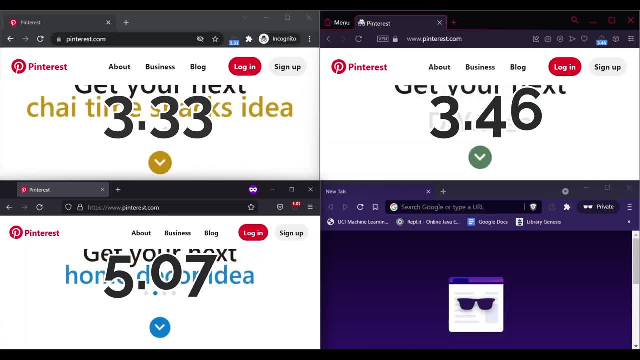 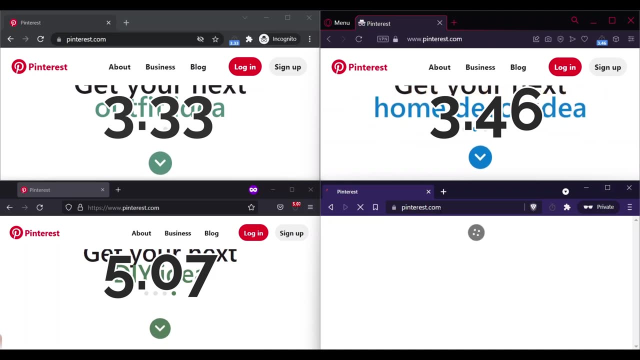 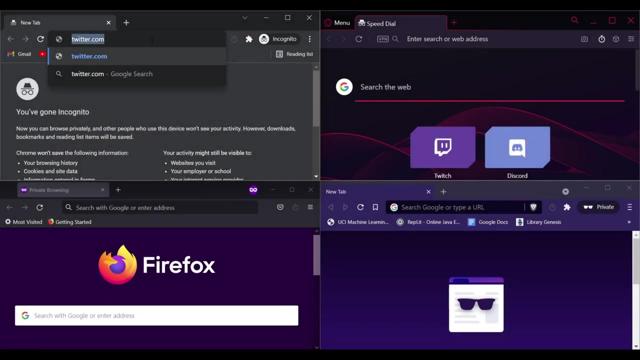 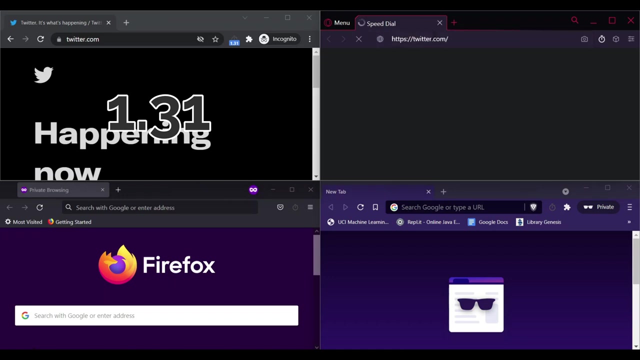 Firefox loads in 5.07 seconds And Brave loads in 10.15 seconds. Chrome loads in 1.31 seconds. 80% of the software loads in 1.3 seconds. Google Chrome loading is very fast. Google Chrome loading is very fast. 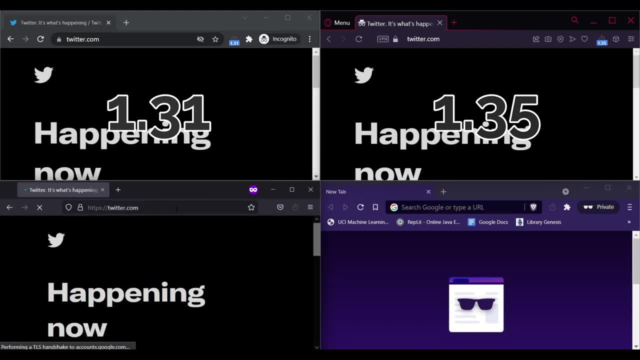 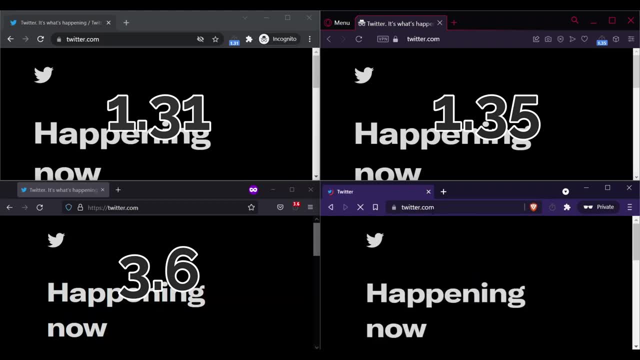 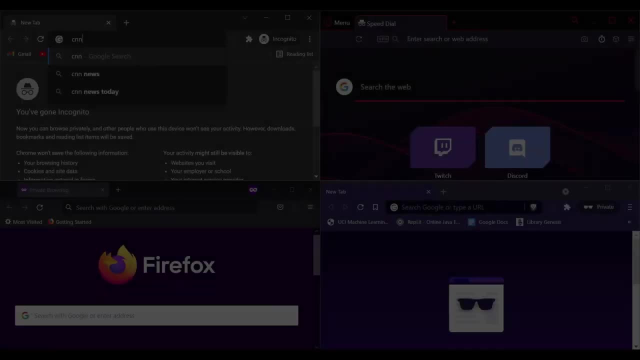 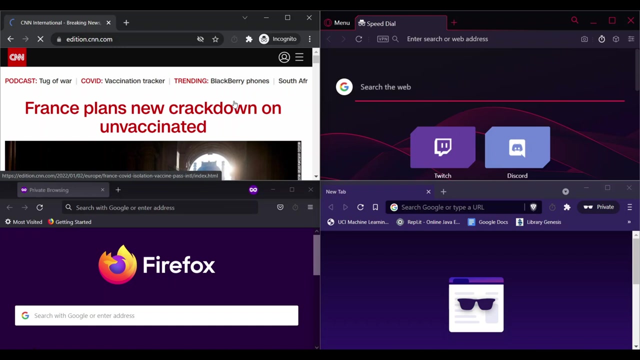 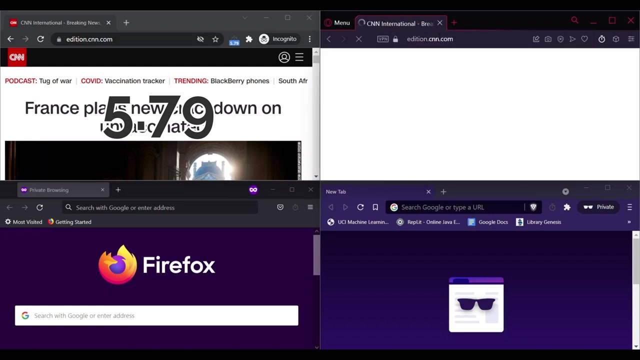 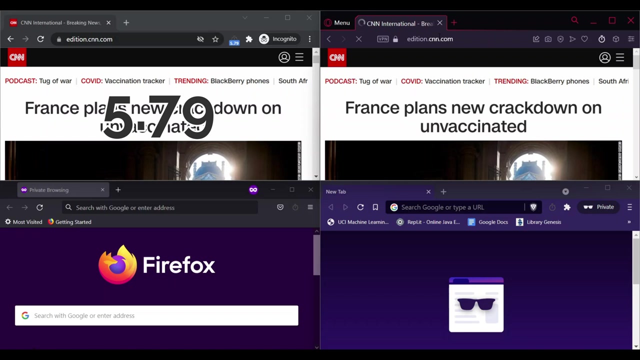 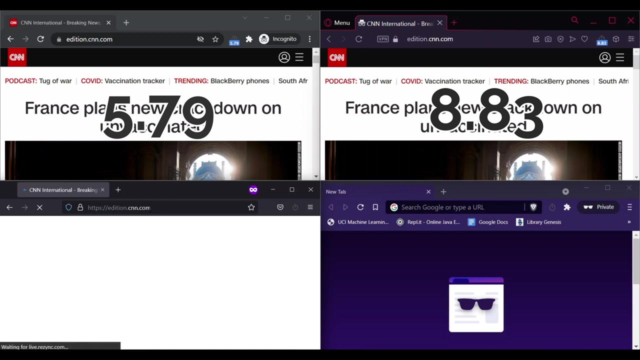 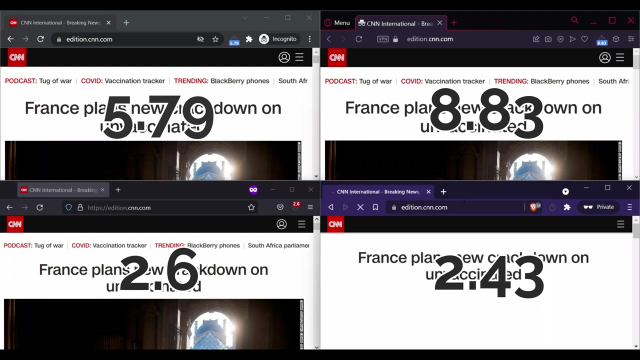 Four different browsers. Firefox loads in 3.6 seconds, Brave loads in 3.07 seconds. Chrome loads CNN in 5.79 seconds. Opera loads in 8.83 seconds. Firefox loads in 2.6 seconds And Brave loads in 2.43 seconds. 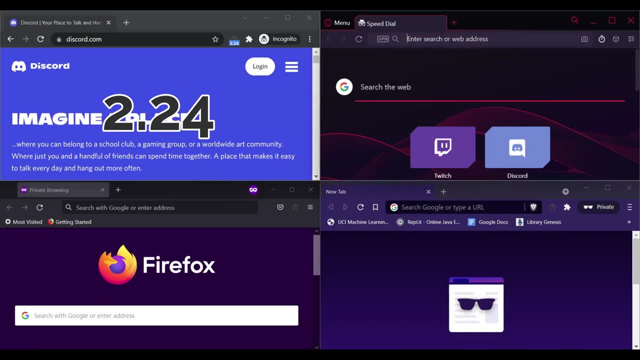 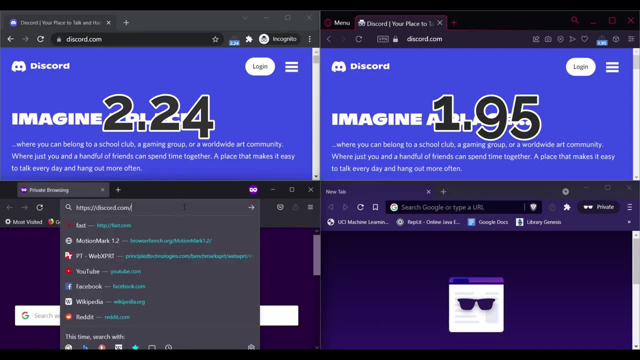 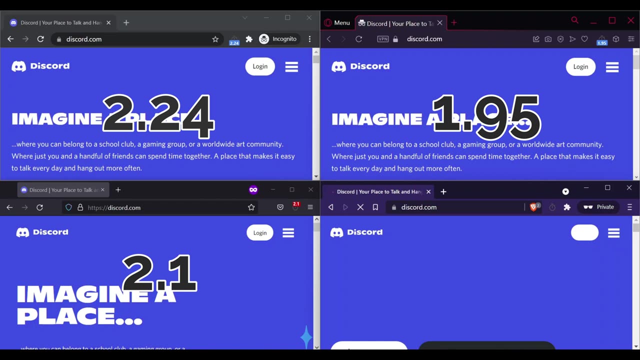 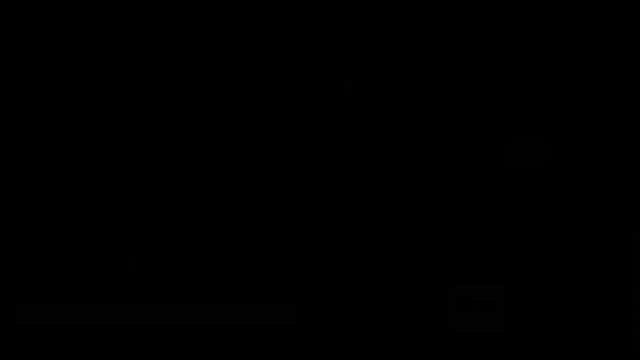 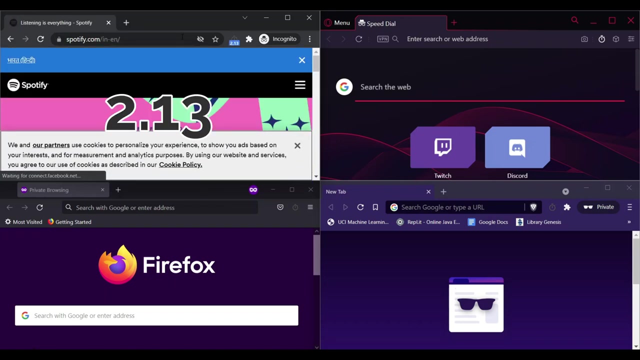 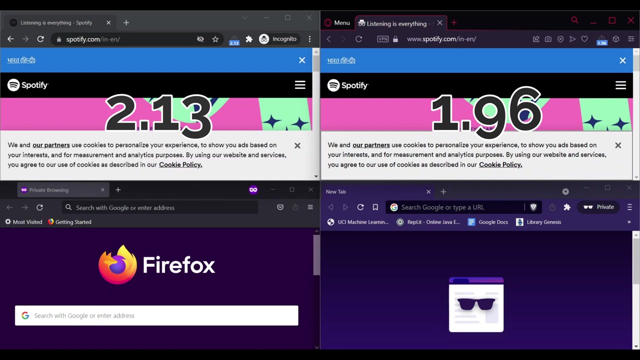 Chrome loads Discord in 2.24 seconds, Opera loads in 1.95 seconds, Firefox loads in 2.1 seconds And Brave loads in 1.95 seconds. Chrome loads Spotify in 2.13 seconds And Opera loads in 1.95 seconds. 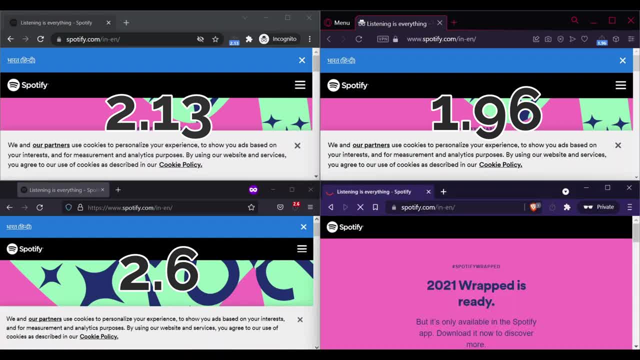 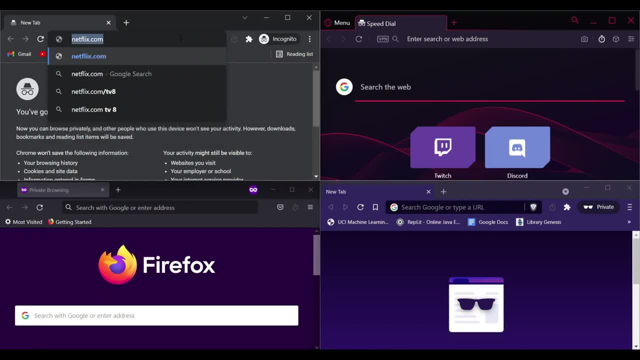 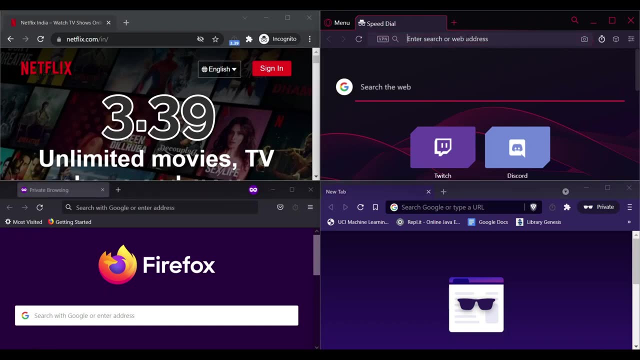 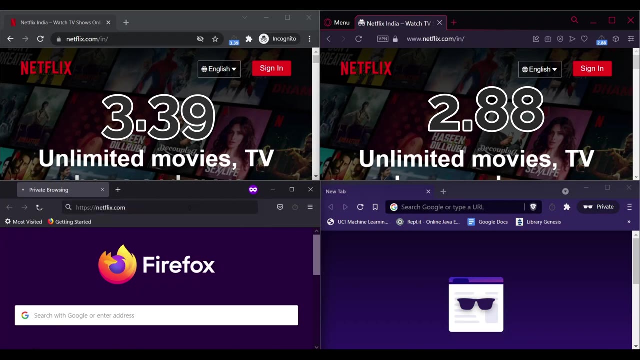 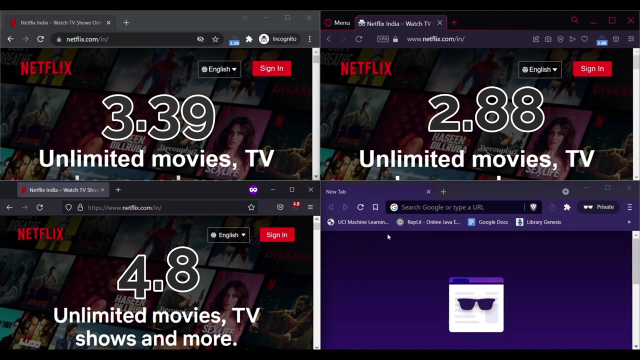 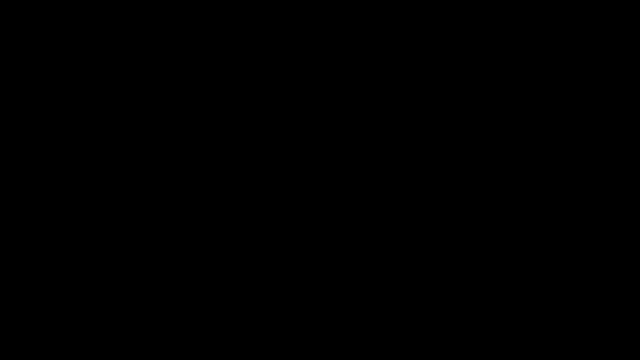 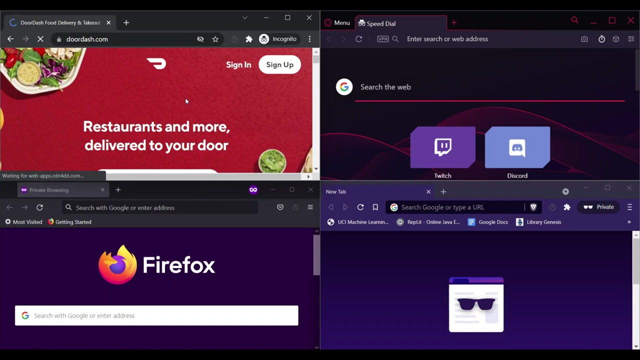 Firefox loads in 2.6 seconds And Brave loads in 1.5 seconds. Chrome loads Netflix in 3.39 seconds. Opera loads in 2.88 seconds. Firefox loads in 4.7 seconds And Brave loads in 2.81 seconds. 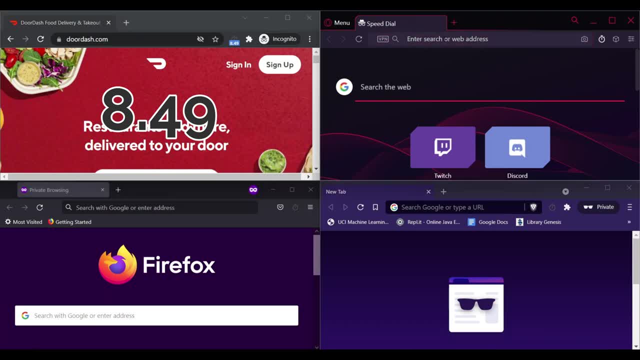 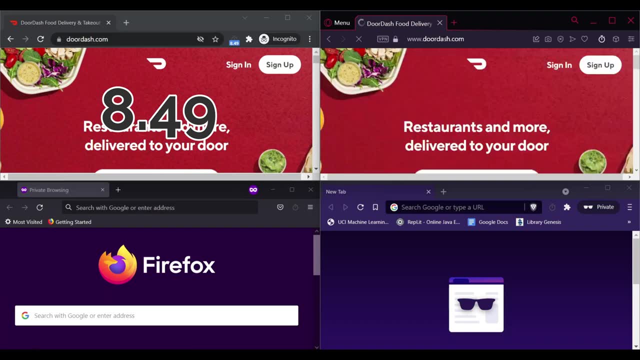 Chrome loads DoorDash in 8.49 seconds And Chrome loads Windows in 2.9 seconds And emetery And OneNote And Microsoft And Google And Mac And Kimmy And John uh And nicole. 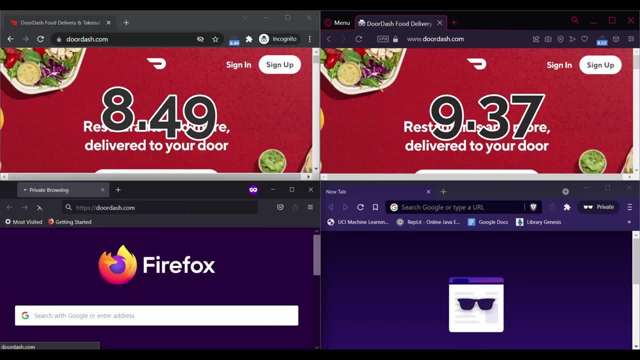 And Michael And Armand, Andミー And And Steven And Billum And everyone else. Then it comes to Freedom Key Instagram too. But These are f'n very mourning things. Everything is. These are f'n very comforting things. 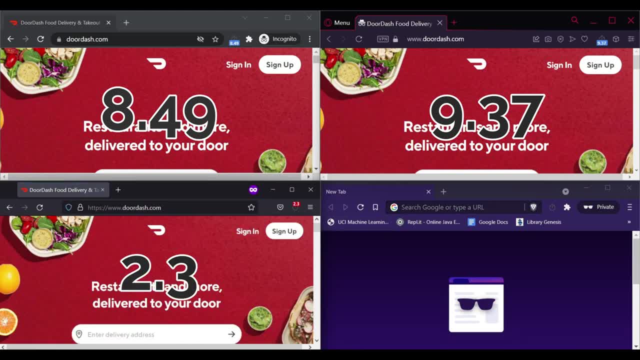 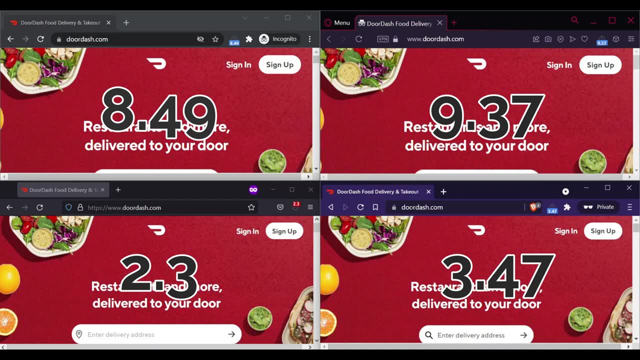 But far too many, kindly. It's time Paul's PDF is in here. You never know when the files will get stung. uuuuuuurrrr For all the people who pay $4,000 for Google around the world. Learn a little Spanish. a little bit about the office mark in chatzzle.